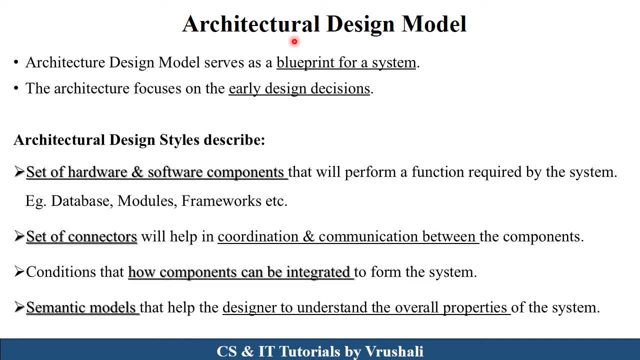 So in this particular project there are different modules, users, functionality, data structure, Components, program database, features, Right, So everything have mention in one diagram. This is called as architectural diagram. This diagram, also called as blueprint of system, Means how your product look like in future. These all things have mention in one diagram. 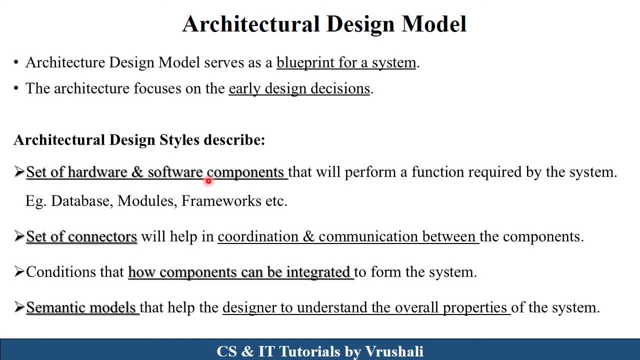 softwares, database, modules, frameworks are there, so everything have mentioned in one diagram. they also mention the coordination and communication between all the modules and the components. basically, they mention complete data flow, complete workflow of particular product and the project. this semantic model help designer to understand overall properties and functionalities in 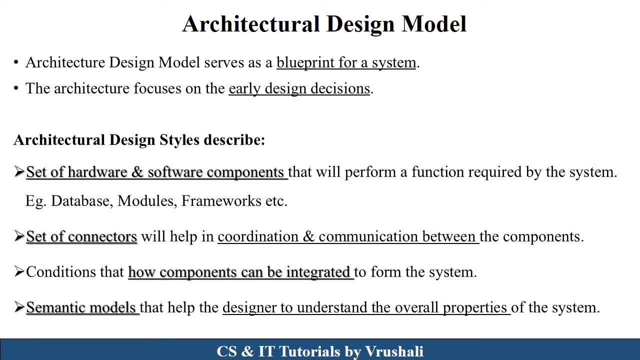 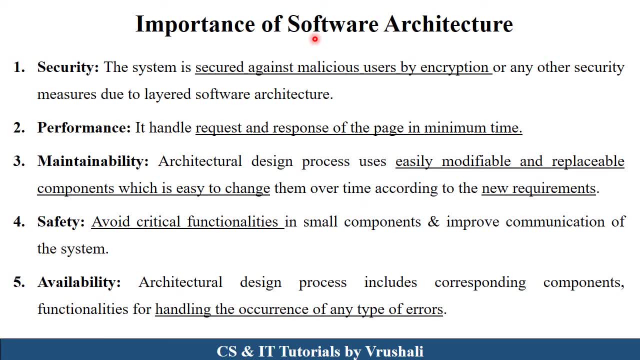 particular system. this architectural design model sent forward to the developer team for development purpose. the next thing is importance of software architecture. the software architecture generated in this way that they provide the security towards your product. they mention in design different login credentials, authentications like OTP, this- all types of features. that's why they secured your. 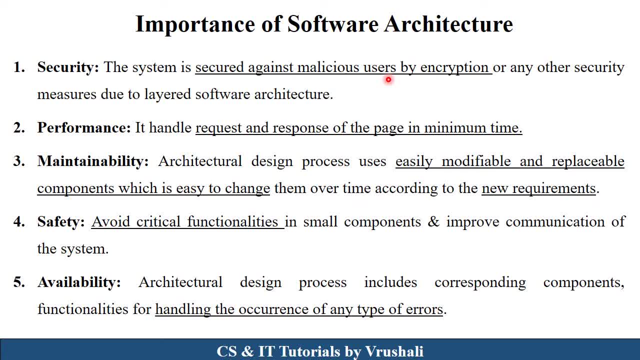 product against malicious users and different types of viruses. software architecture also handle the performance of your product. they handle request and response of page in minimum time. the best example is Google search engine. you can search on Google and they show the result within a second. right now. software architecture also easy to modify and replaceable components, because customer 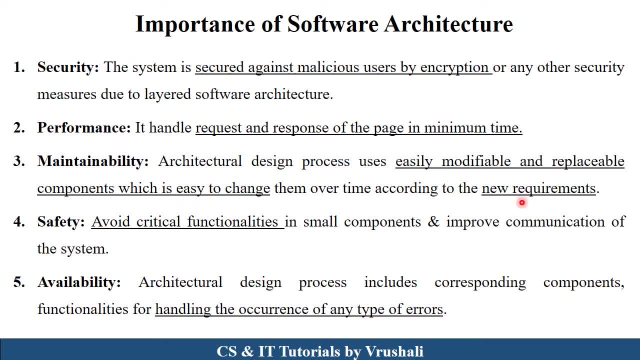 requirements are continuously changing so they can easily modify a particular components, features, in particular Product software architecture also provide safety towards the customer. they generate a particular product as per the customer requirement and customer safety related features are there. software architecture also handle different types of errors, components and the 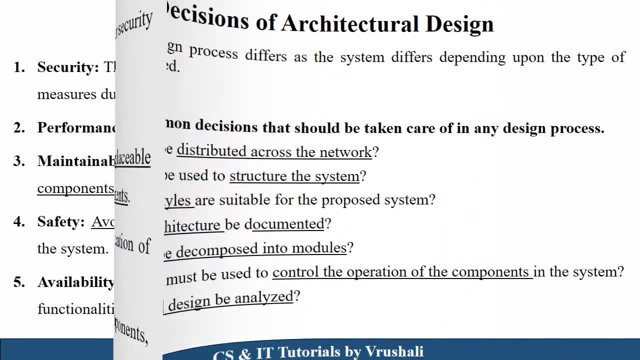 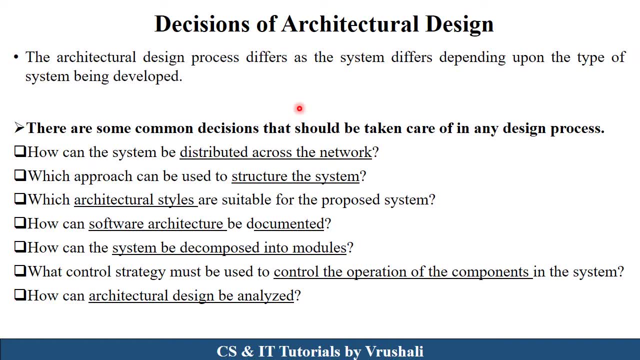 complete flow of system. the next thing is decisions of architectural design. see, there are different types of software applications. apps are there, right, in daily life you can use banking application, online shopping application than gaming application or reservation applications, social media applications, right. so every app having different architecture, different. 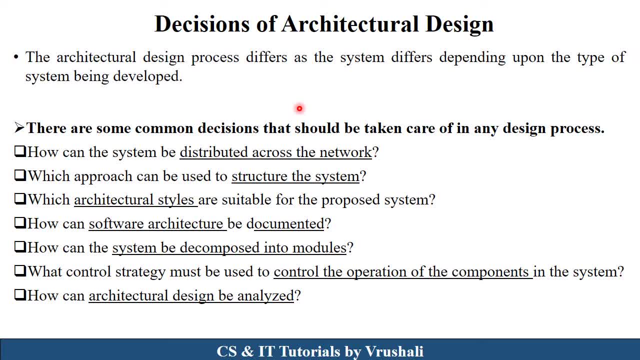 functionalities are there, right, but still there are some questions that will be helpful for each and every software applications before generating a design here. designer discuss some types of questions. designer discuss how can the system be distributed across the network. they discuss that the particular product used at state level, country level, international. 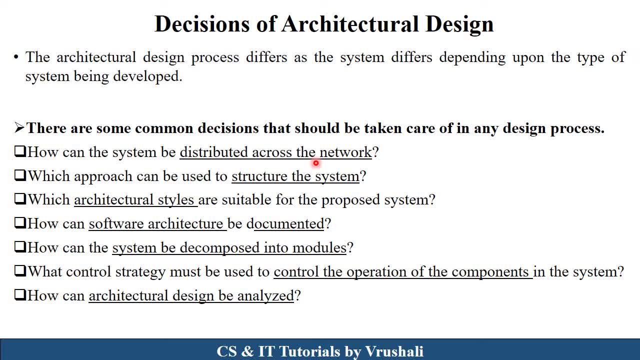 level or particular organization level. they understand the distribution of particular Network designer also discuss complete structure of system, architectural style, then software architecture documentation. then which type of modules are there then control of operations, how each and every components are interrelated with each other? so this, all questions have decided. 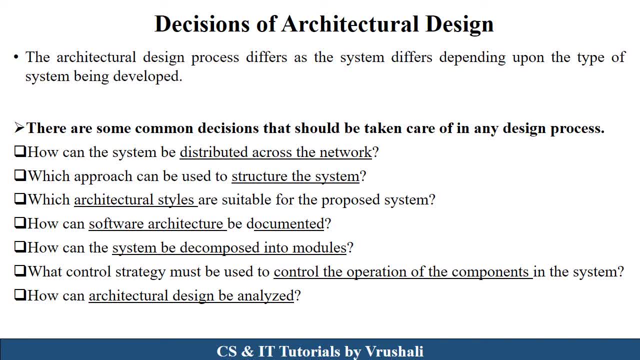 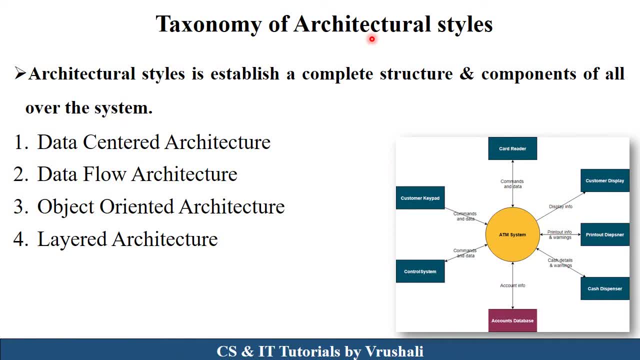 and after that they take a decision For generating a architectural design. the next topic is taxonomy of architectural style. as exam point of view, this- all types of architecture- is one of the most important question. there are four types of architectural style: data centered architecture, data flow architecture, object-oriented architecture and layered architecture. 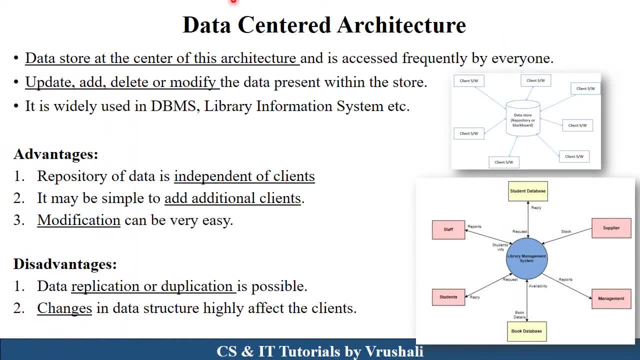 let discuss one by one. the first type of architecture is data centered architecture. the name suggests that data-centered architecture has stored at center place. for example, see here in this diagram. this is a centralized data right and multiple user access those data at the same time. this is called as data centered architecture. 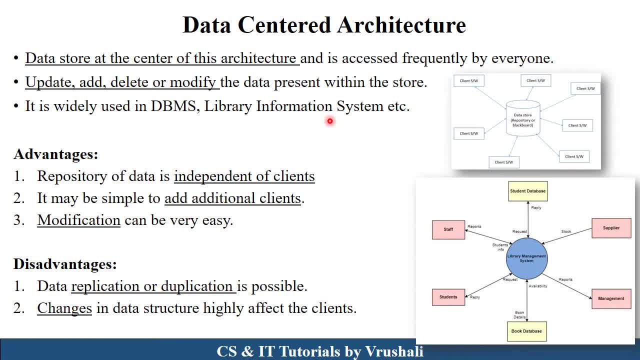 generally this data centered architecture concept used in particular organization in DBMS, in library information system like this: see here in this diagram. this is a library management system database and there are different types of users, like student database, supplier, management book database, then a staff, so everyone perform. 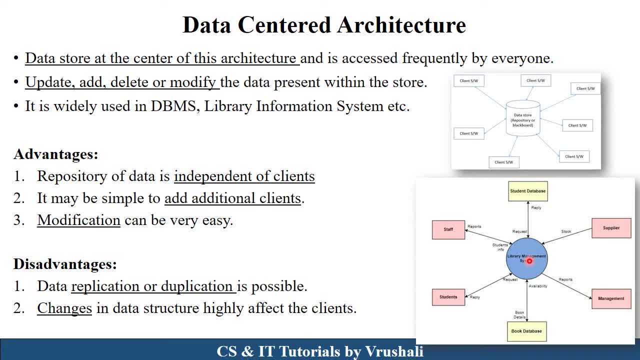 the particular action on this database as per the requirements. right, they perform update, add, delete, modify- this kind of operations on the same database. this is called as data centered architecture. the advantages of data centered architectures are there are independent of clients. means every user perform action as per the requirements. 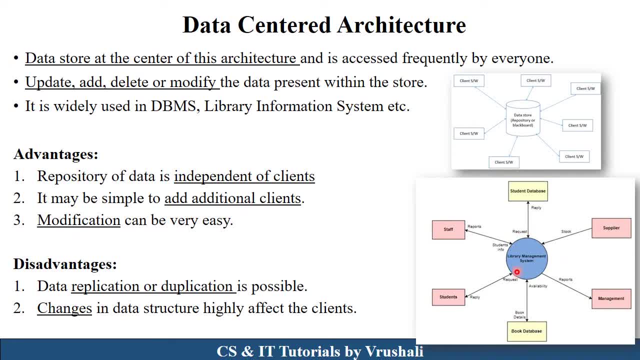 it is very simple to add additional clients Here: librarian add additional students and staff. It is very easy to add the different users. then modification also easy in the particular database. but the disadvantages are data centered architecture. They perform every operation at the same time. 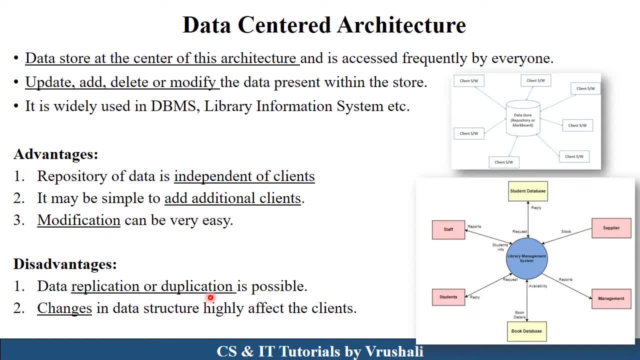 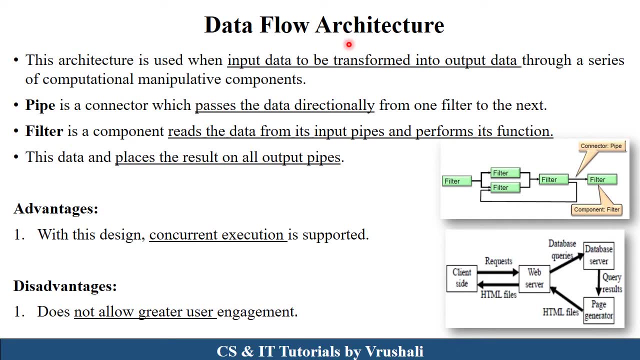 That's why there are duplication values have generate and changing in data structure is effect on client because they perform update, add, delete at the same time, right, So this is called as data centered architecture. The next type of architecture is data flow architecture. The name suggested, data flow, means they handle a complete input data. 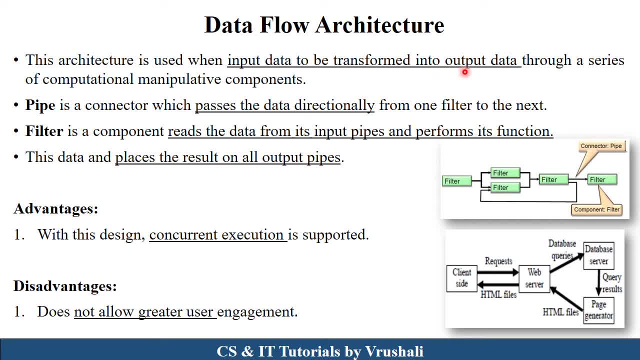 that to be transferred into the output data flow of particular product. see here in this diagram: here this all lines, this connectors are called as pipe and this filter are called as components. So this show the flow of complete system. pipe is a connector. They passes data directionally. the directions have show. 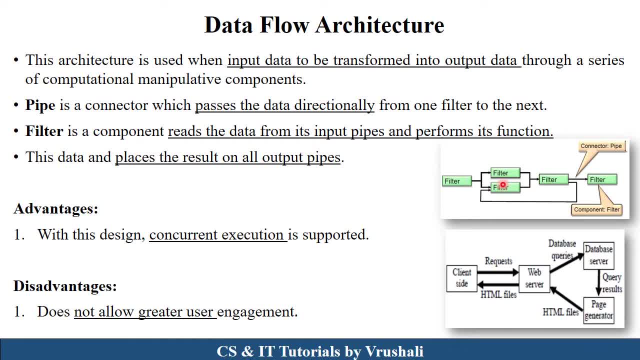 That is, input to output form, and filter means there are different actions, different functions, different manipulations have performed in this particular filter component. The best example of data flow architecture is Google search engine, see client search. something on Google, for example: client search, software engineering tutorial. then this request sent to the web. 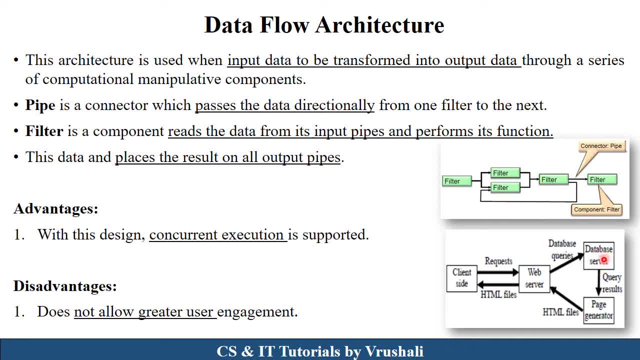 server. web server check this query in database. then database display different types of software engineering tutorials towards the customer right miss particular data flow is there. This is called as data flow architecture. The advantages of data flow architecture is there is a concurrent execution is supported. means from client side request web server web. 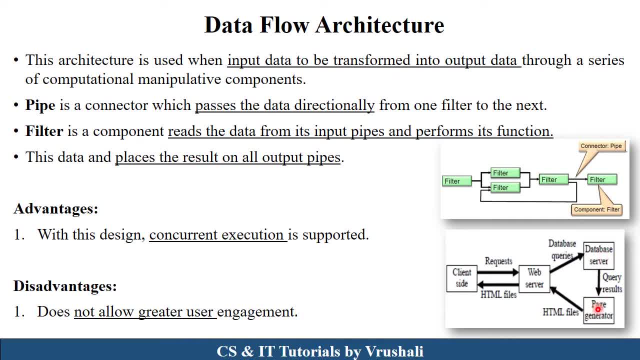 server request database server. database server display result. again, this result show to the client right miss. there is a. concurrent executions are there, but the disadvantages are. that does not allow greater user engagement. The best example Of this: see when your result was declared. so all students search. 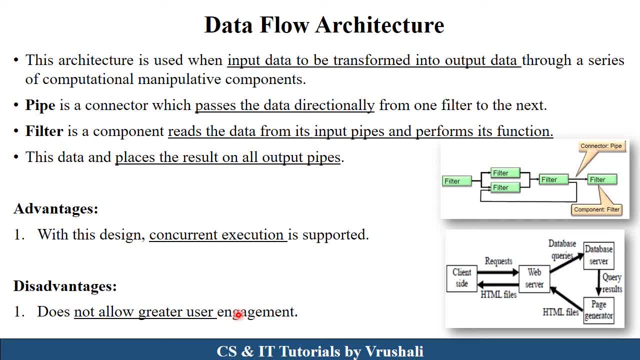 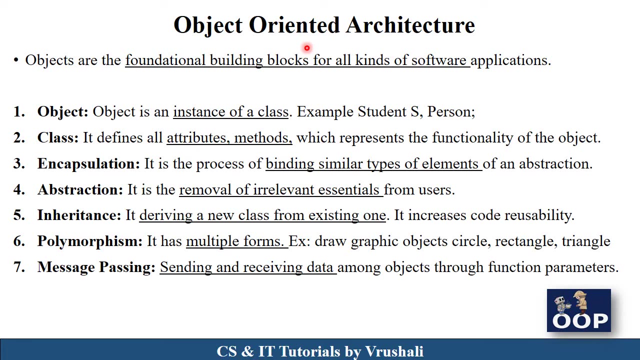 a particular result site, your university site, right? or sometimes this particular website get hang because multiple users engagement are there, right? or same thing happen with your scholarship websites, right, so they does not allow greater user engagement. This is called as data flow architecture. Now, the next one is object-oriented architecture, so basically object. 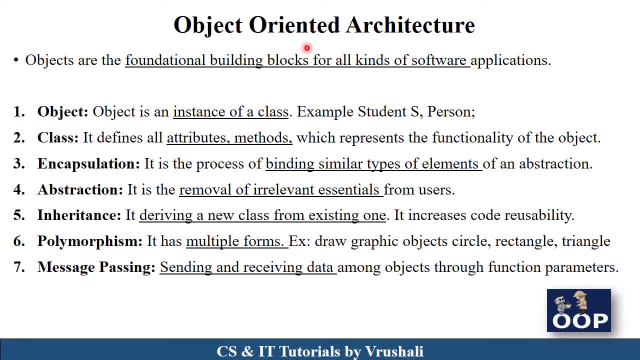 oriented architecture is foundational building block of particular software. This is a base. This is a foundation of your particular product. I think you already learn OOP subject where you can learn this- all types of concepts and term. So these all terms are necessary while designing or developing a. 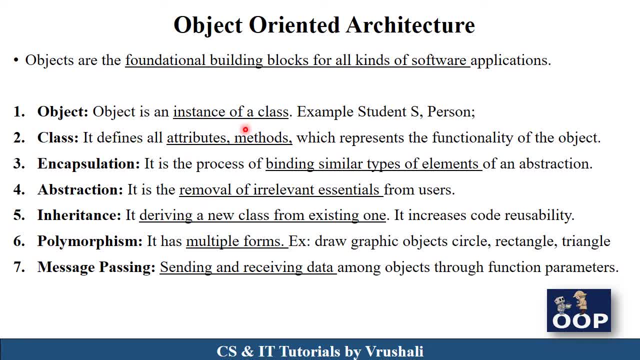 particular product. So object. object means instance of class. There are student, person, company, So this kind of objects are used as per the project requirement. then class, color. class means collection Of different types of attributes. methods are there. encapsulation means the binding, similar types of element, similar types of data, like student, 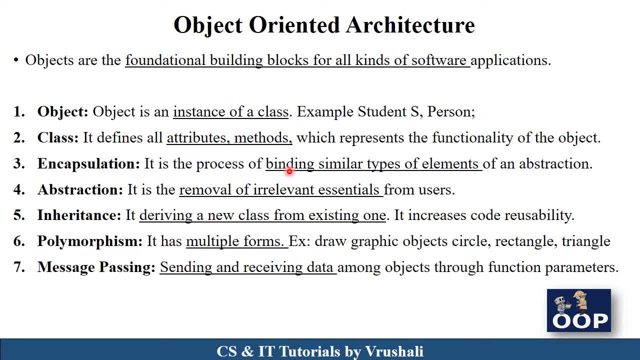 marks in one encapsulated, then student gaming information is there. then student awards are there. This, all things are called as encapsulation. abstraction means they remove irrelevant, essential details from the user. They show only required information to the users. inheritance means there are a parent and child relationship. is there right? 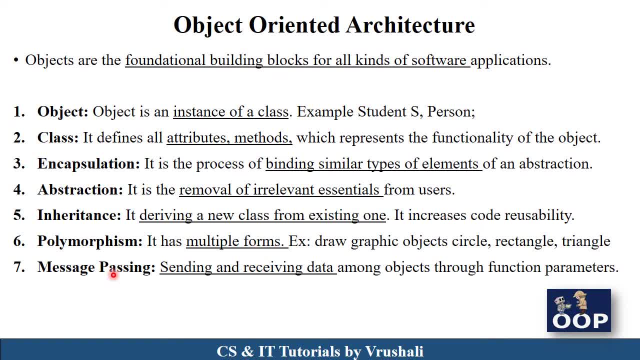 Then polymorphism- There are multiple forms are generate and message passing means sending and receiving data through the object in particular product. So these all concepts are used for generating, developing and designing a particular product. This is a base of complete software application. Now the next one is a layered architecture. 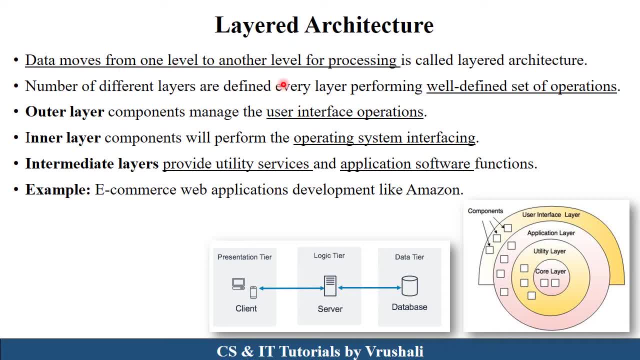 So layered architecture. here data move from one level to another level for processing purpose, which is called as layered architecture. See here in this particular diagram. The outer layer is user interface layer. For example, user interact with particular software. user use WhatsApp, So they use their front end functionality, front end interface only. 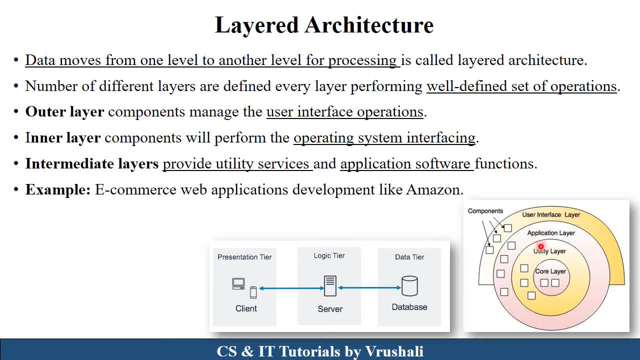 right. So this is a user interface layer, but intermediate layer. there are application layer, utility layer. application utility layer means which is related to the server, like HTTP, HTTPS, and core layer, Related to the programming database, means there are particular layered architecture. is there right? 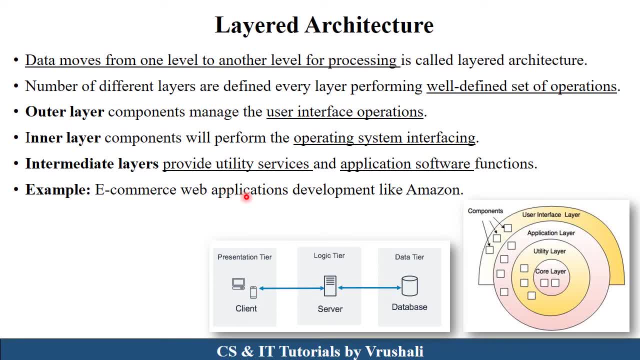 The best example of layered architecture is e-commerce web applications development like Amazon, Flipkart or Google search engine. These are the best example of layered architecture. See here in this diagram. here clients search something on internet means the server is there, So server access those information from this database. database give the 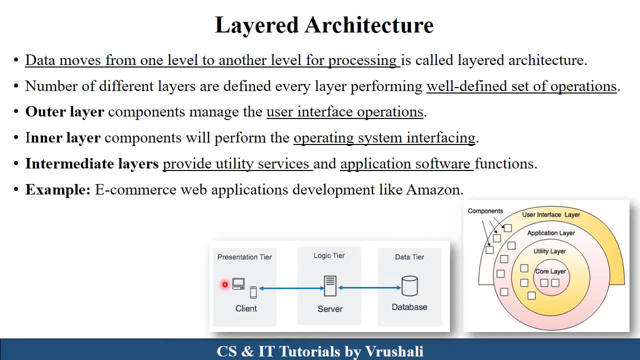 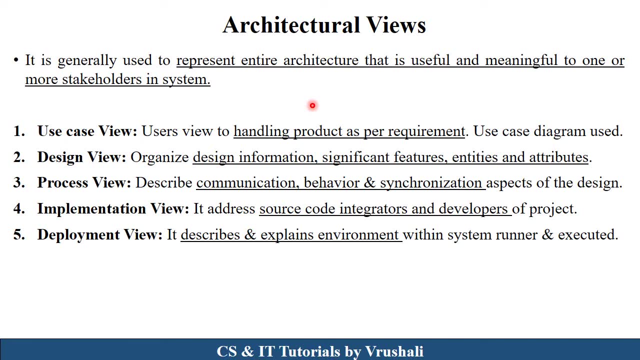 result to server. server Give the result to the client. right me, There is a particular layered from presentation logic to data layer, right. So this is called as layered architecture. Now, the next point is architectural view. Now there are different types of architectural and database designs. 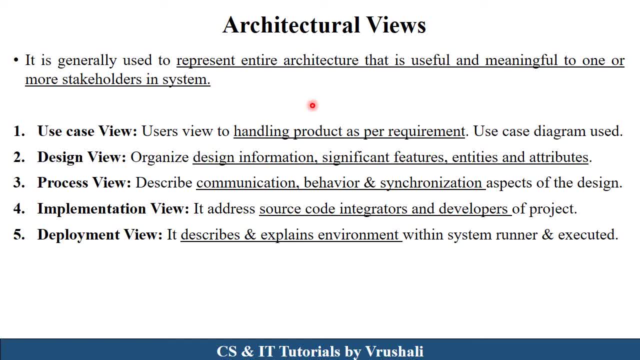 are there right. So there are different stakeholders, different users use those architectural diagram. but there are different views of particular architectural design. The first view is use case view means how user use a particular product. This is a one type of view right. user use a particular product as per. 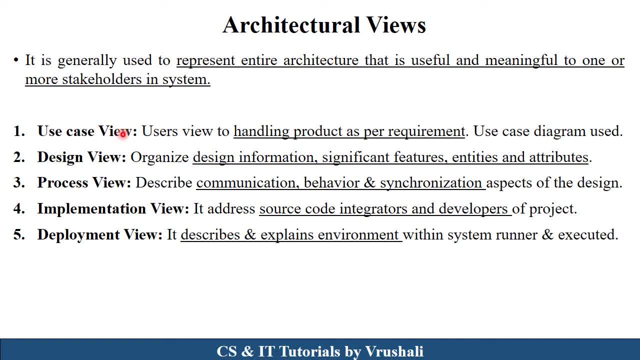 the requirement, right. So this is called as use case view. use case diagrams are used. Next one is a design view. design view means which type of components are placed, means which type of text- box, button, checkbox, radio button- So everything have placed in one particular form, right? 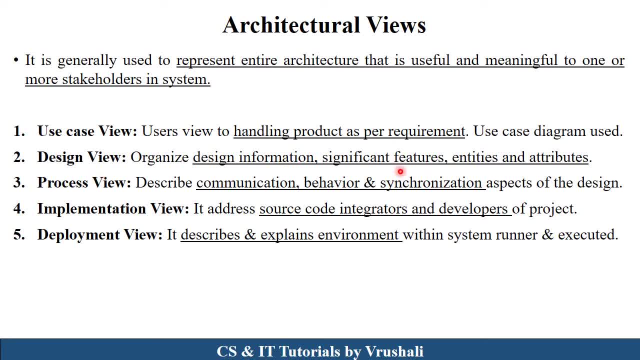 So this is called as design view. They show the information, features, entities, attributes in one particular form. then process view. process view means the flow of system, the communication behavior between different modules, different applications. when you click on submit button, the next page will be open. So this is called as process view: the behavior of particular system. 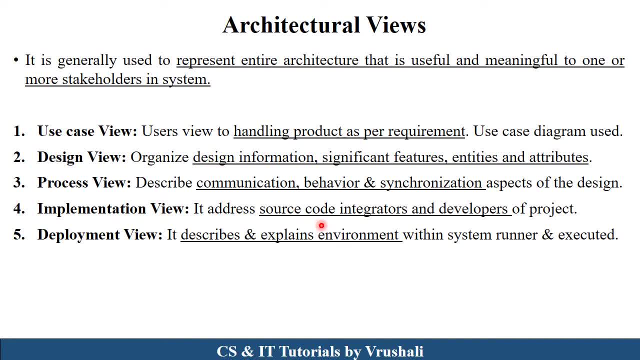 Next one is the implementation view. So implementation view related to the source code developer or particular database related Functionalities. and last one is a deployment view: means after completing your product, your product deployed to the customer environment, for example, college management system application. So after developing this product, this product deployed at a college level.